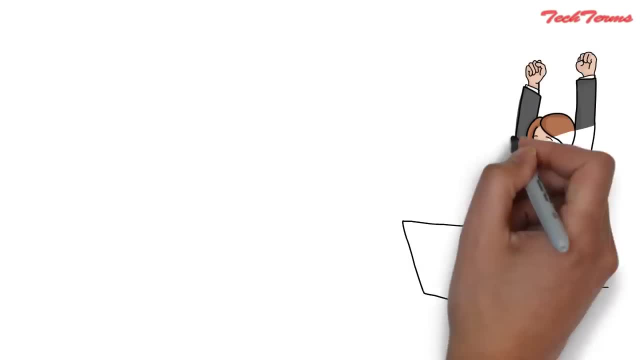 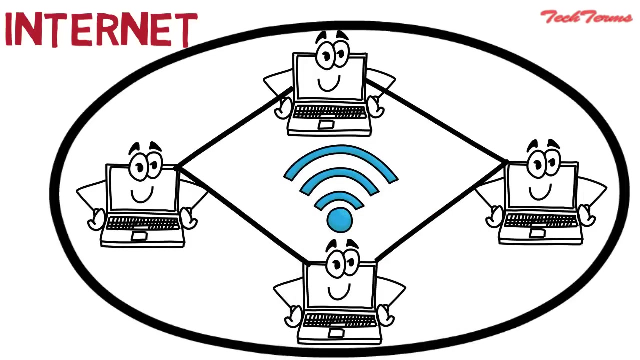 Hey guys, this is DG. Today we are going to understand what is an IP address and how you can find your computer's or your smartphone's IP address. So let's start. Computers in internet communicate with each other with underground or underwater cables or wirelessly. If I want to download a file from internet, then my computer should have. 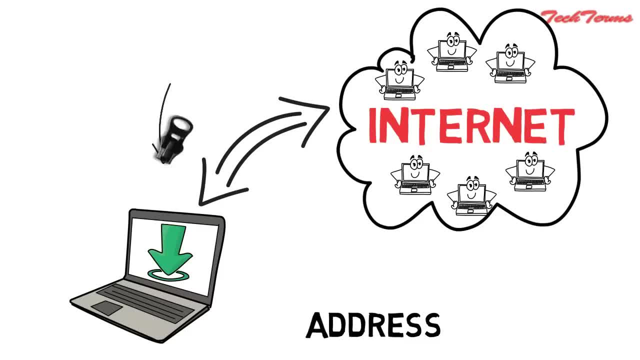 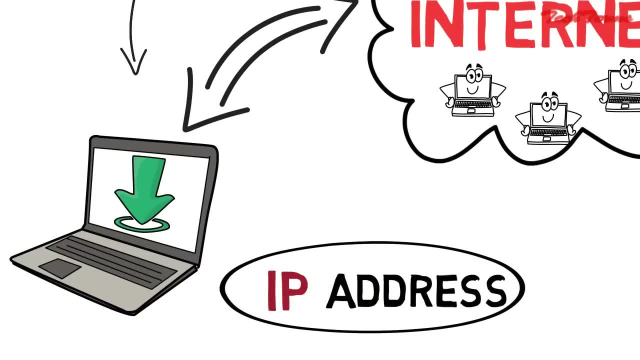 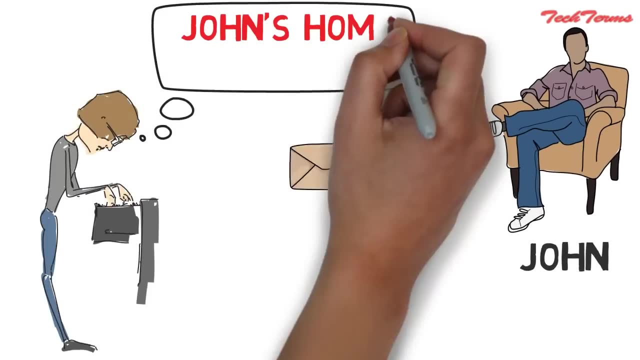 an address so that other computers in internet can find and locate my computer. In internet terms, that address of computer is called IP address. Let us understand it with other example, Like: if someone wants to send you a mail, then he or she should have your home. 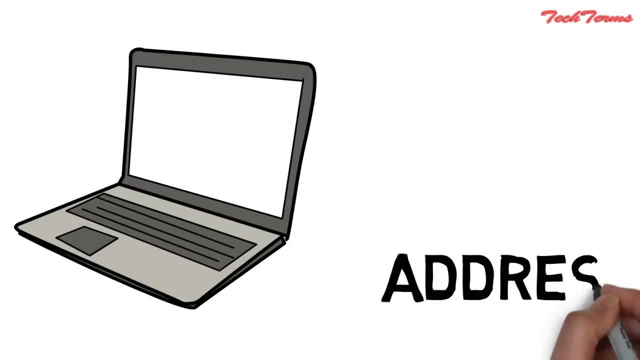 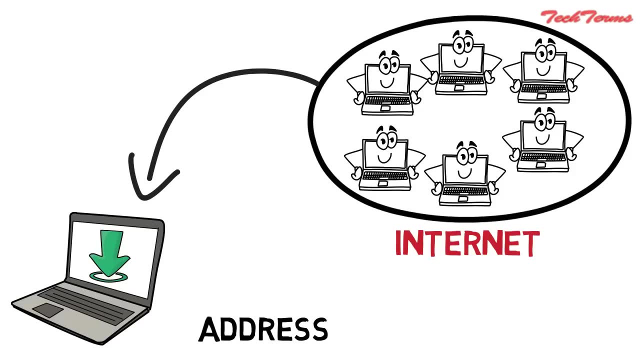 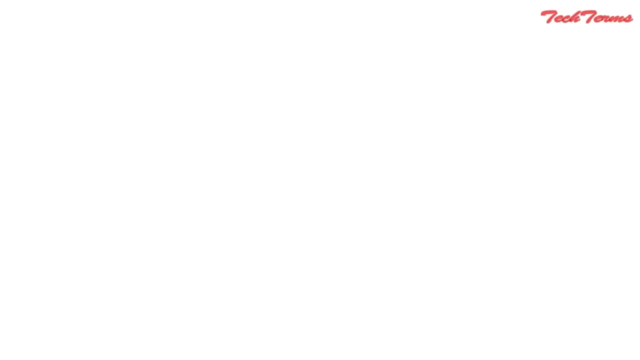 address. Similarly, your computer also needs an address so that computers in internet can send you a file that you want to download. That address, in internet terms, is called IP address, which is nothing but a string of numbers written in a certain format. Note. 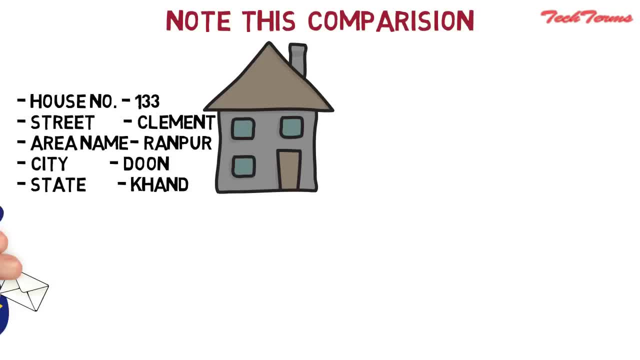 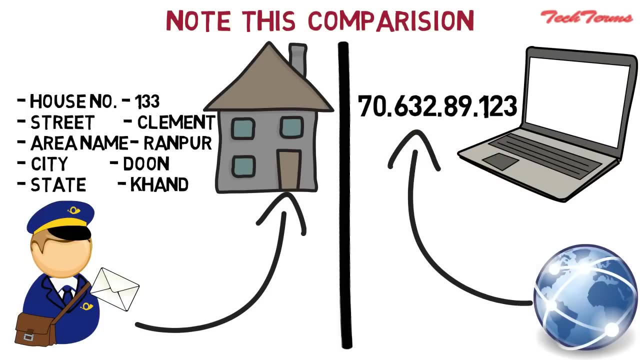 this comparison: This is your home address, which is identified by your area postman, and you get all the things delivered in this address. Similarly, this is your computer address, which is identified by the computers in internet, and you get all the downloads available at this computer address. This address is the IP address of your computer IP address. 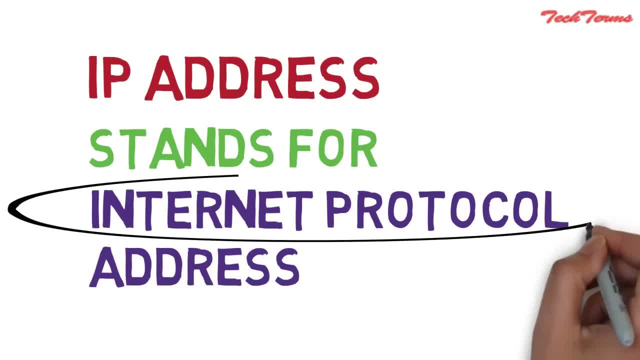 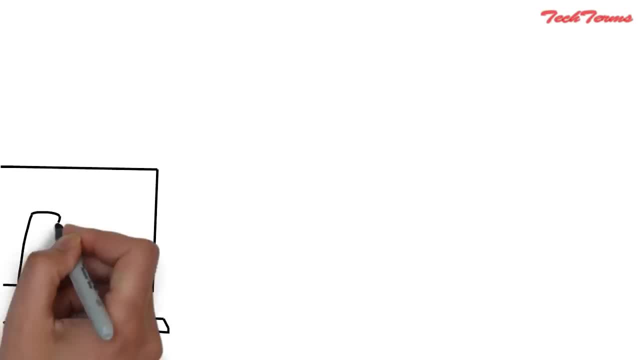 stands for Internet Protocol Address. But what does this mean? Internet Protocols are the IP addresses of your computer. They are the IP addresses of your computer. Internet Protocol is a set of rules that makes Internet work. You are able to watch this video, this time in YouTube, only because your computer or your smartphone. 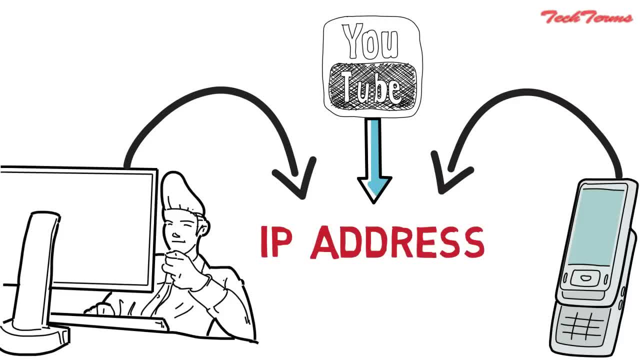 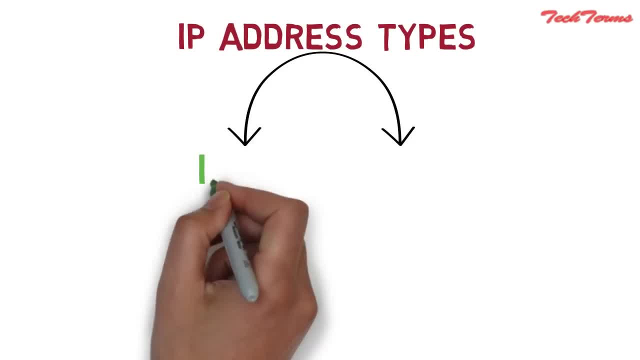 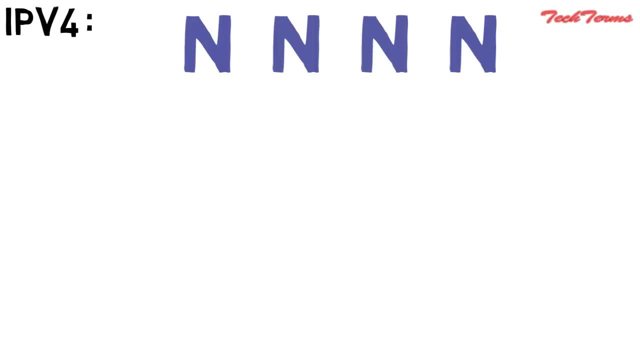 has an IP address and YouTube is sending you all the data related to this video to this IP address. IP address is of two types: Internet Protocol Version 4 and Internet Protocol Version 6.. Internet Protocol Version 4 consists of four numbers, separated with the two numbers. 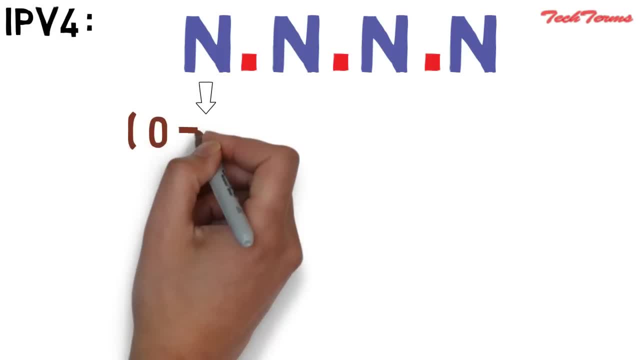 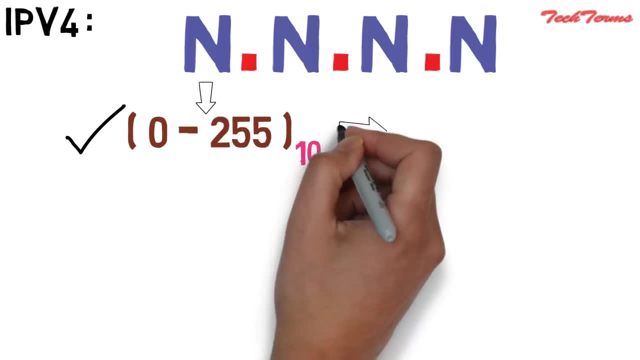 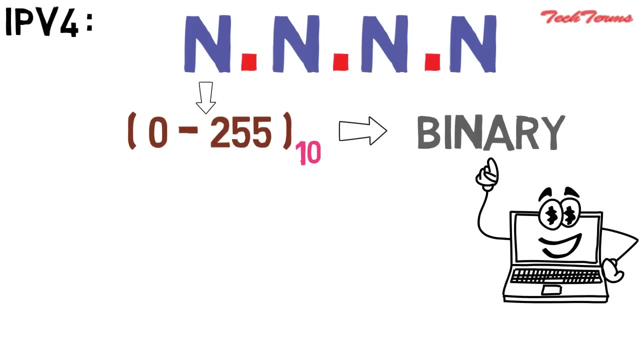 Each number can range from 0 to 255 in decimal numbers, But computers do not understand these decimal numbers, So these numbers are converted to binary form, which is computer understandable. Therefore, in binary, this range can be written as 0000000000 to 11111111.. Since each number 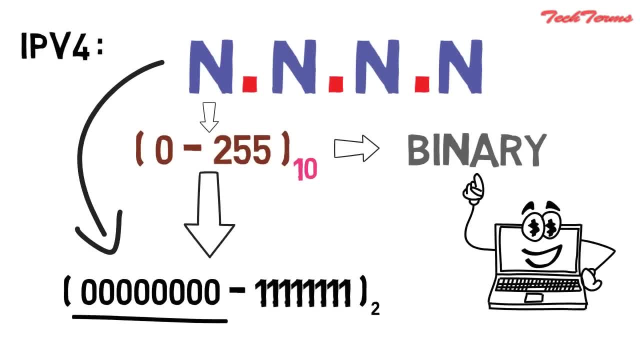 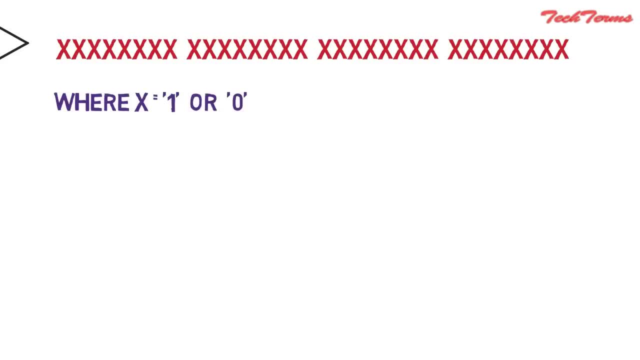 N is represented by a group 1,, 0 and 1 in the IP address. So when you make this kind of group of 8 binary digits, so the whole IPv4 address is represented by a sequence of 32 1s and 0s, or simply I should say by a sequence of 32 bits. 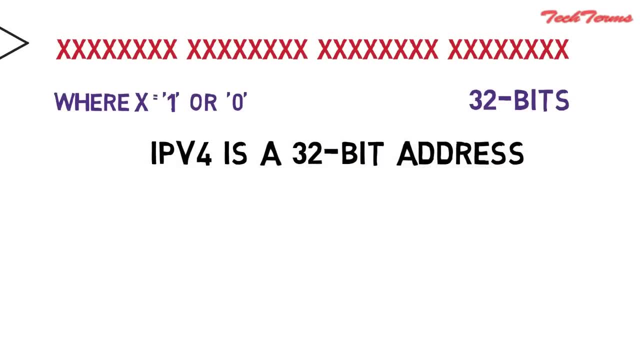 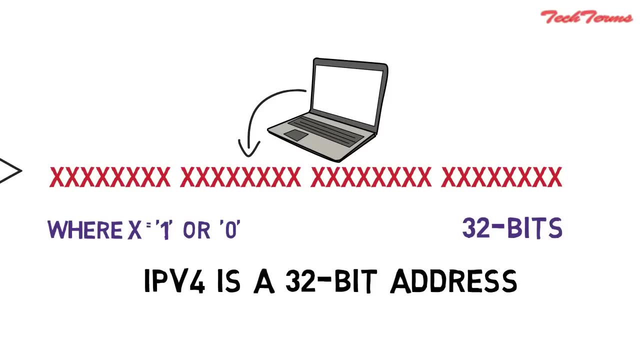 So IPv4 is a 32-bit address. In IPv4, a unique sequence of 1s and 0s is assigned to each computer. Therefore a total of 2 raised to power 32 devices, that is approximately 4 billion devices. 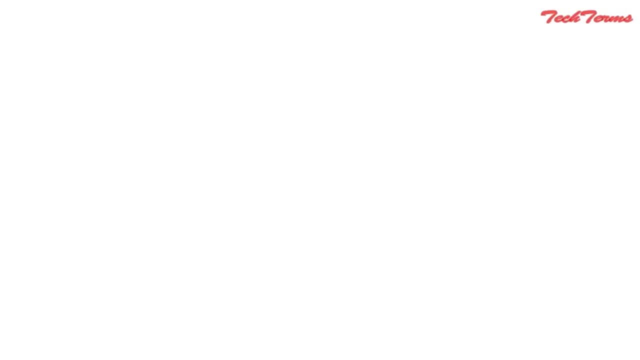 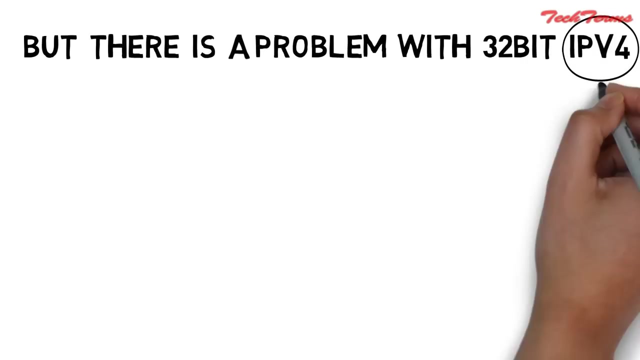 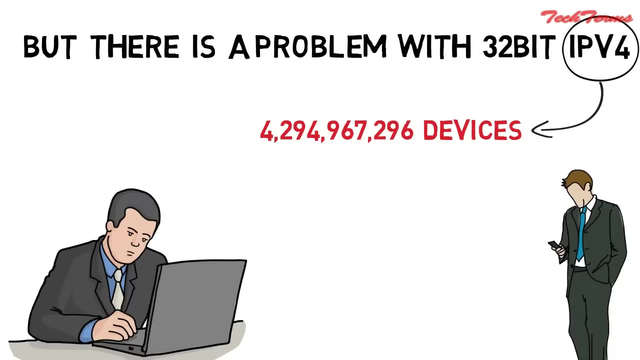 can be addressed and connected to internet with IPv4. But there is a problem with this 32-bit IPv4 address. With IPv4, we can connect only this amount of devices to internet, But these days we have devices like computers, smartphones- far more than 4 billion. 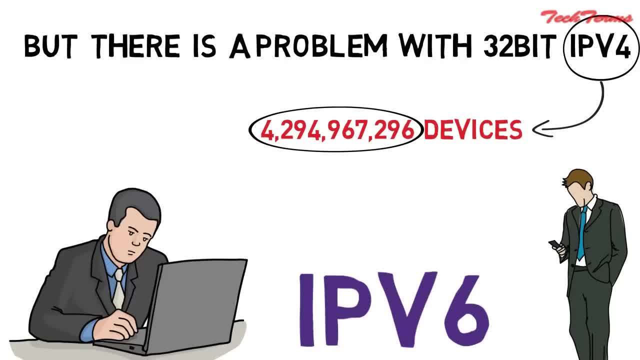 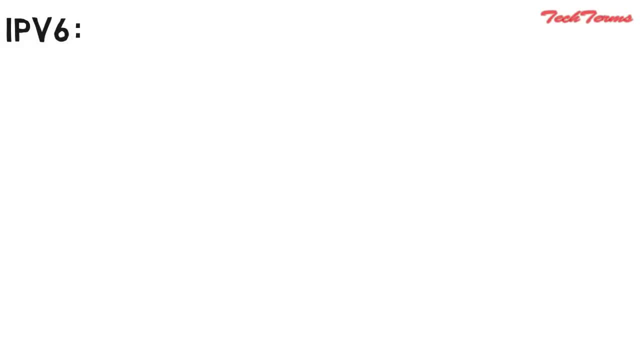 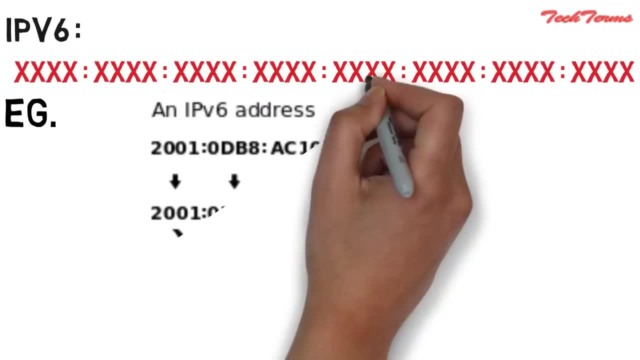 So slowly we are moving towards IPv6.. IPv6 address is a 128-bit IP address. In human-friendly form, IPv6 is written as a group of 8 hexadecimal numbers separated with colons. For example, in human-friendly form, the IPv6 address can be written like this: 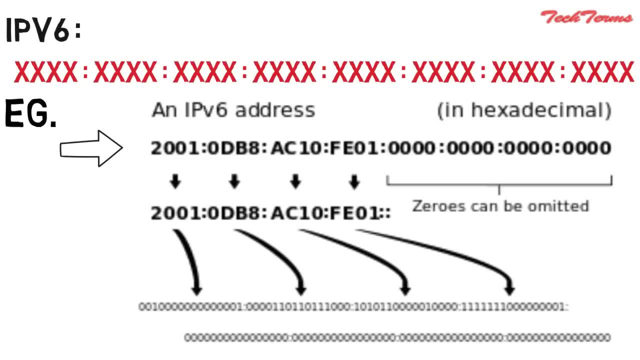 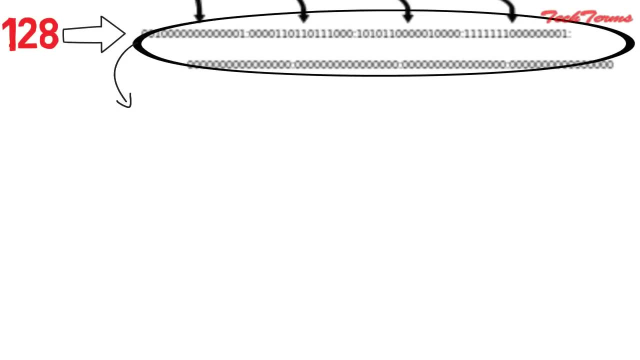 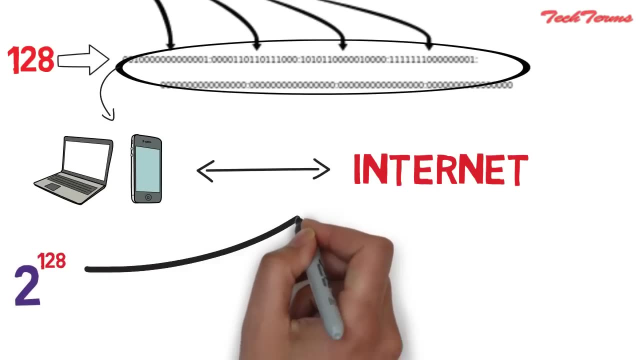 While in computer-friendly form, IPv6 address can be written by a sequence of 128 1s or 0s, Since a unique sequence of 1s and 0s is given to each computer, So with IPv6, a total of 2 raised to power, 128 devices can be connected to internet. 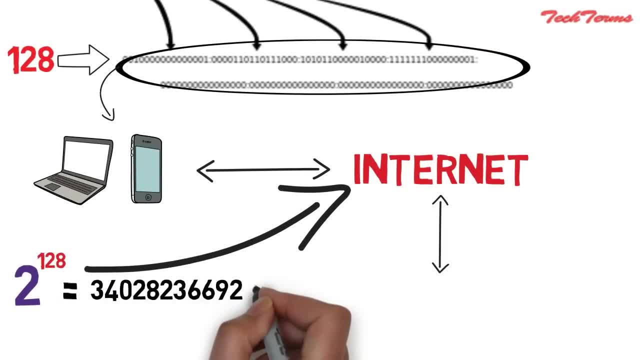 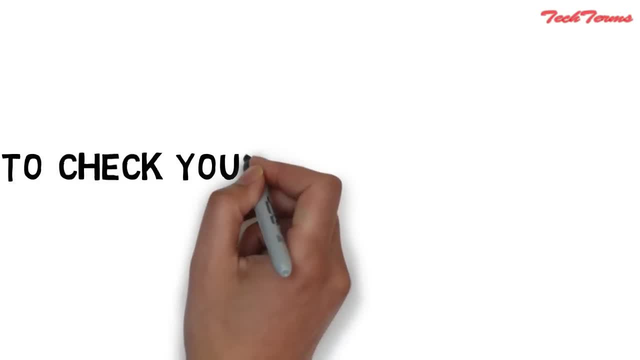 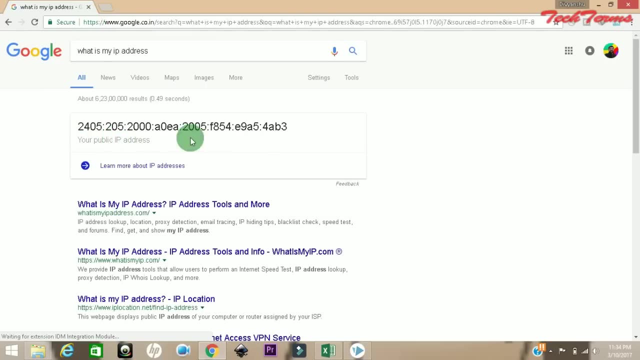 That is, IPv6 can address this amount of devices, which is actually far more than enough for many future generations. To find your computer's public IP address, write what is my IP in wwwgooglecom. Google will tell you your computer's public IP address. 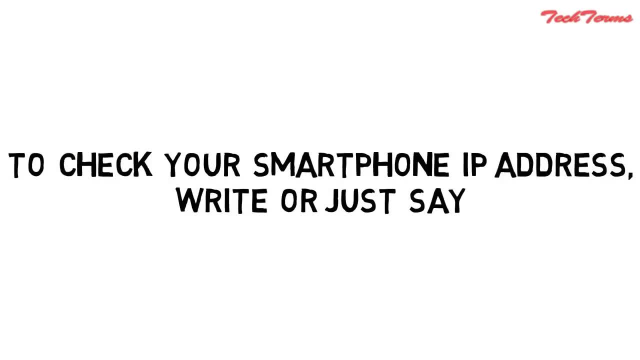 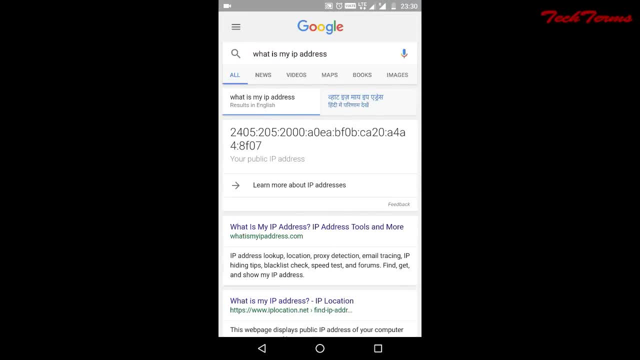 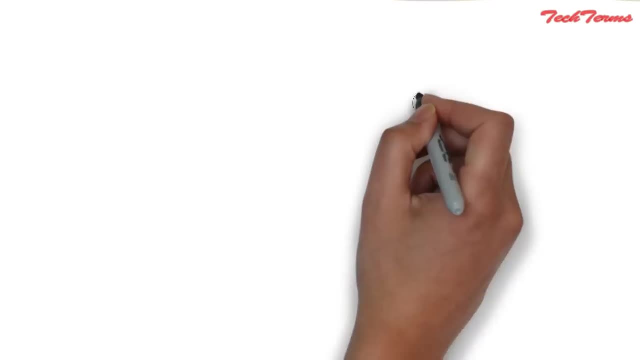 Similarly, To find your smartphone's public IP address, write or just say what is my IP in your smartphone. Google will tell you your smartphone's public IP address. Without this numeric protocol, we would not be able to connect to internet, And without internet we would be standing in long queues to get our train tickets. we 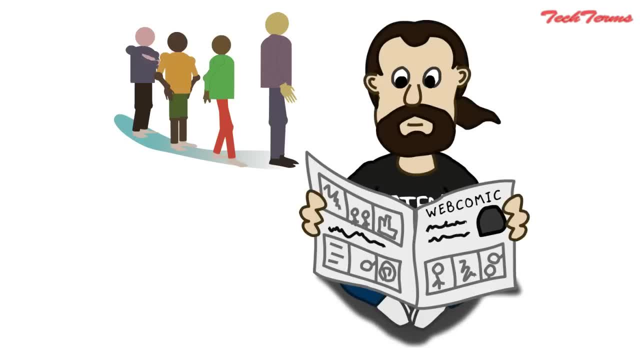 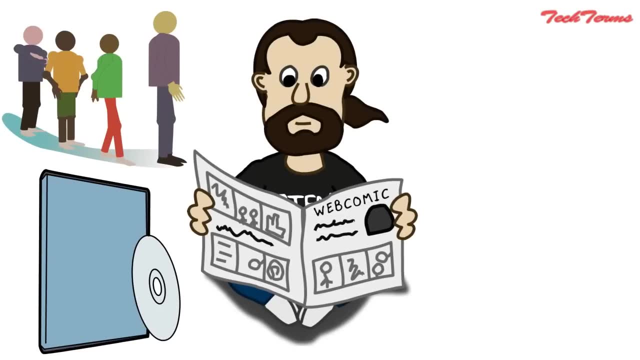 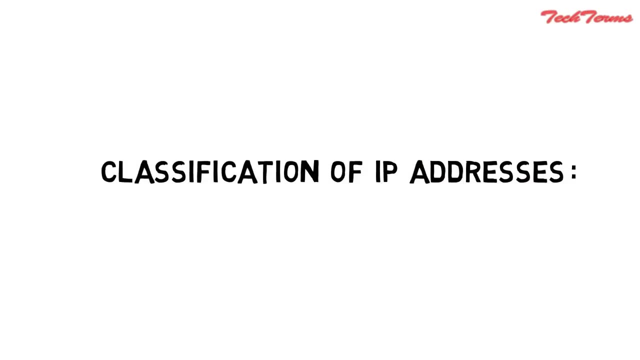 would be looking at newspapers to see where jobs are available, and we would be buying storage devices like CDs, because without internet, cloud storage would not work. So IP address is must for internet connection. IP address can be classified as dynamic IP address and static IP addresses. starting.